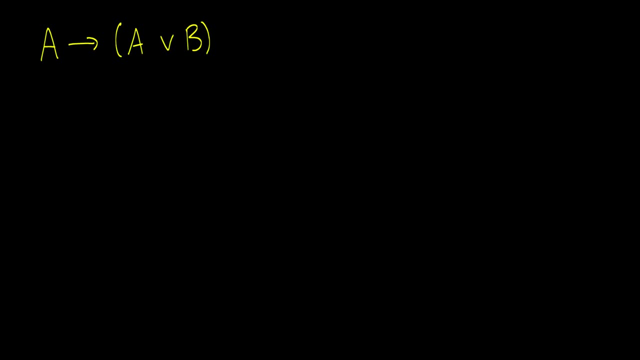 tautology or contradiction. but I want to ask you specifically: is this a tautology? So a reminder? a tautology says that all outputs are true. So what we can do is, instead of having to draw a whole truth table, 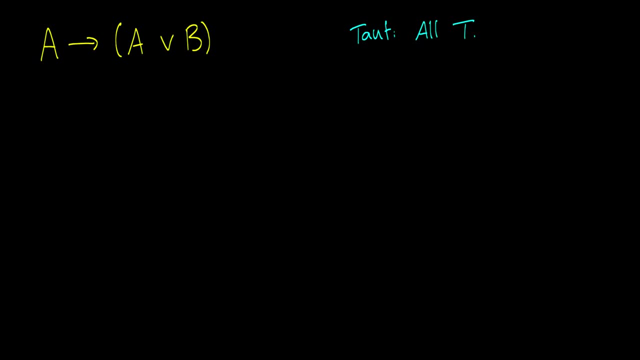 why don't we just say: well, let's just suppose the sentence is false. Okay, so we suppose the sentence is false, And now what we have to do is we have to create truth values that make it false. So we know, an arrow is only false when the antecedent is true and the consequent is false. 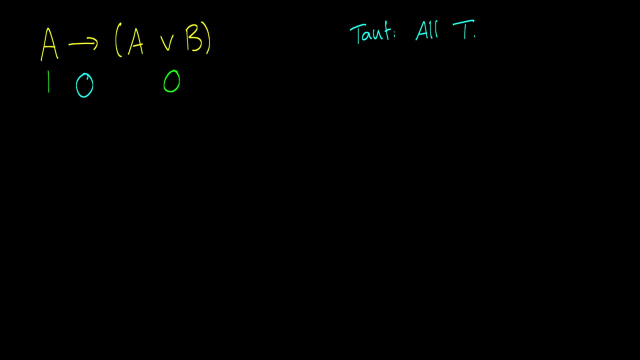 And a disjunction is false only when both of its disjuncts are false. So now from this we can make a claim That there is no possible output that is false. And if you remember I have one is true and zero. 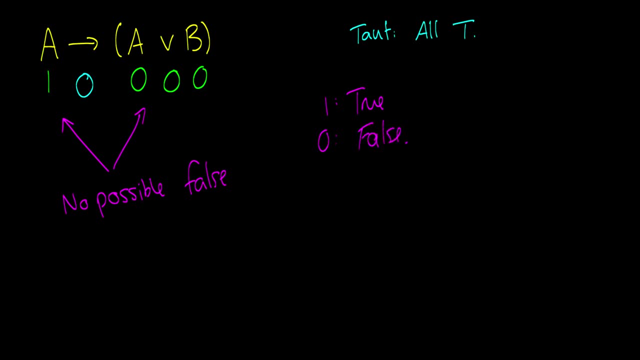 is false. When doing this sort of thing, I like to use zeros and ones, because there's a very clear difference between a t and an f, And sometimes my t's and f's look like each other and they get confused. So because a is equal to zero and a is equal to one, I'm going to use a t and an f. 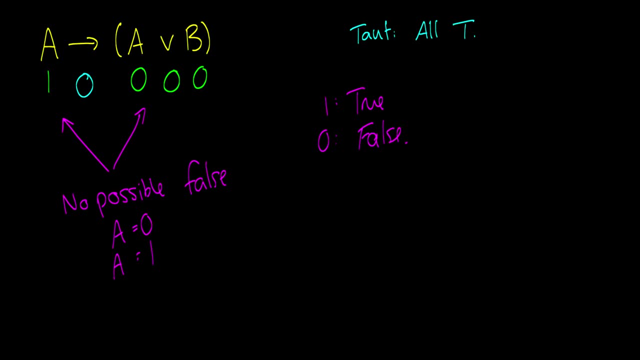 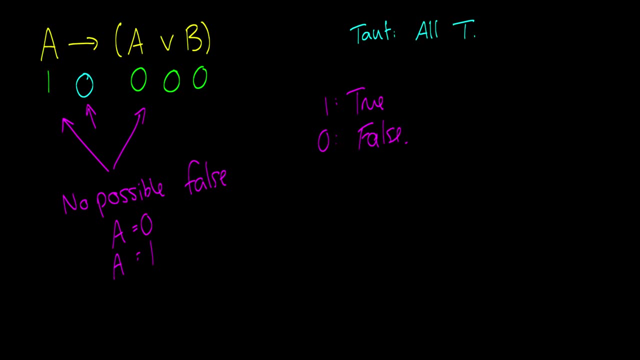 false. Therefore it's its ontology, And I'd like you to try this one real quick, because you know, just just see if you can make this false. I want to see an assignment where this is false, And if you can do it and show me an assignment that's true, and if you can do both, then what? 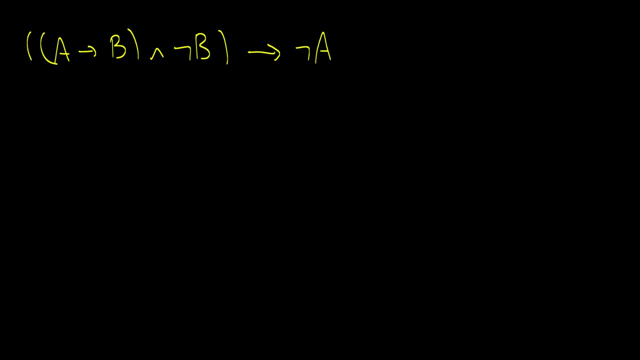 does that say? So? Solve this. just pause the video. I'll just be back in a second. Okay, so let's make this false. So it's going to be false, which means a has to be false. I mean not a has to be false. 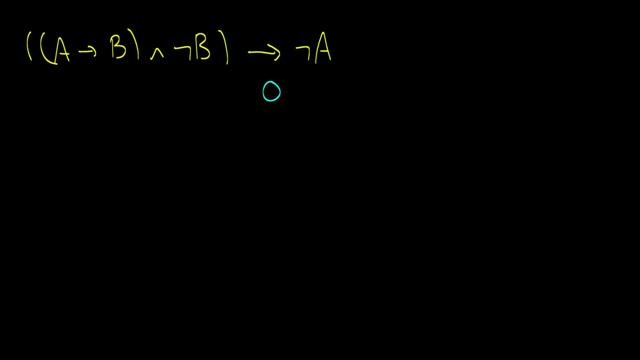 but the whole consequent has to be false, so not a has to be false, which means a has to be true and the left side has to be true. but where are we going to write this? Well, we're going to write this here at the conjunction, because it's the main connective on the left. 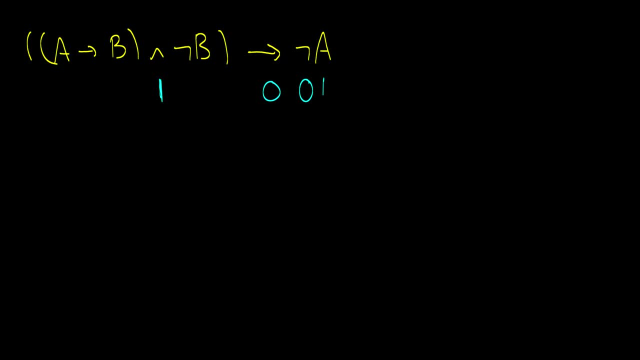 Okay, and if the conjunction is true, then both of our conjuncts have to be true. So we have not. b has to be true, so b has to be false, so b is going to be a 0, so I'm going to write these down here: b is a 0, and we know a is a 1, so let's write this down here. 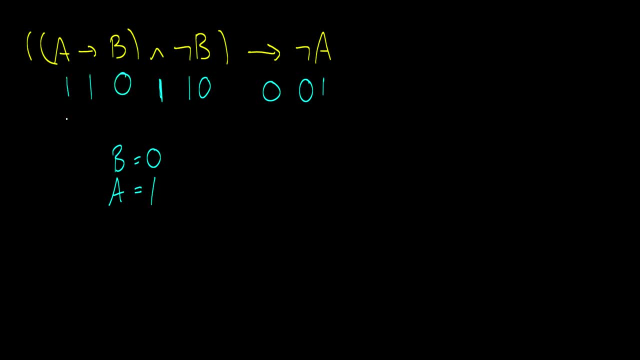 Well, a has to be 1 and b has to be 0, but hold on a second. then that means that that should be false, because the arrow isn't true when a is true and b is false. So again, we have another contradiction here, right there. so therefore it is a tautology. 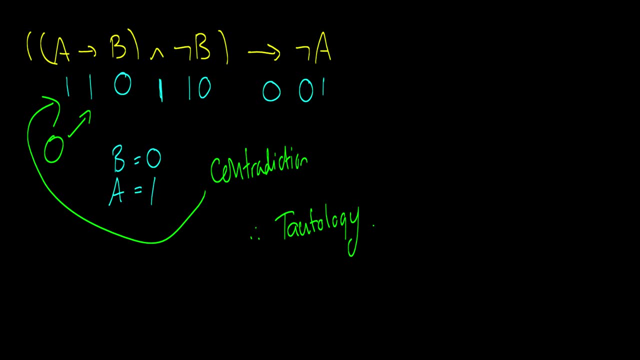 and it is a tautology, because there is no possible assignment where this is true, where the whole sentence is false. So you can do the same thing for finding contradictions, as you can try to make an assignment that's true and realize you can't. 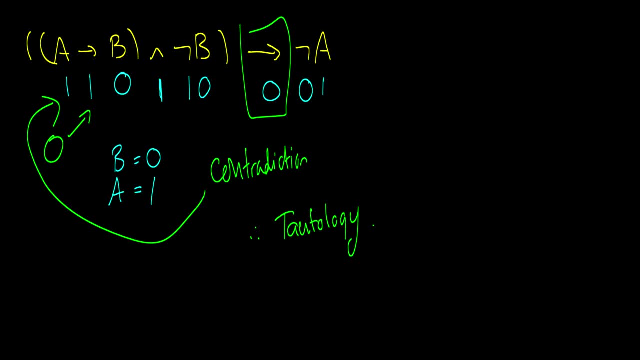 and with contingencies, you'll be able to make one that is true and one that is false. so that is how you figure them out, without doing full truth tables, which is an advanced tactic that is much more efficient and something that computers do pretty easily. 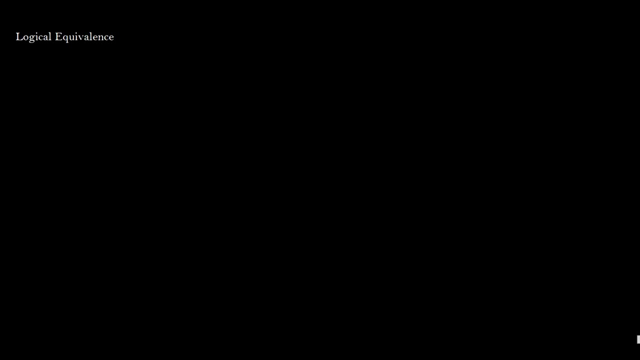 So there's one more thing we need to talk about, which is logical equivalence. and we say two formulas are logically equivalent if they have the same truth table. So can you think of anything that might have? So we have the same truth tables, two different formulas, and there's a very basic one which I'm going to start out with. 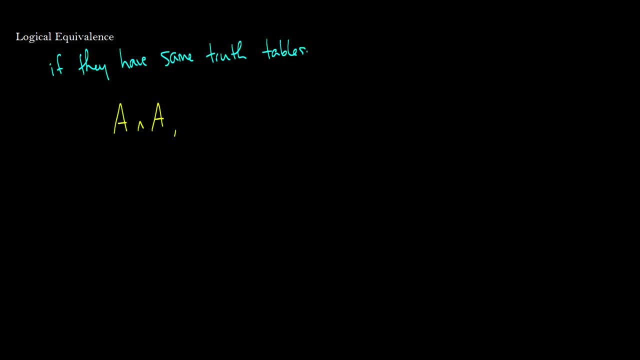 We have a and a, and we have a or a, and we'll just write a here. So the truth table for a is going to be true and false. In fact, I'm going to start using ones and zeros now, because I prefer them. 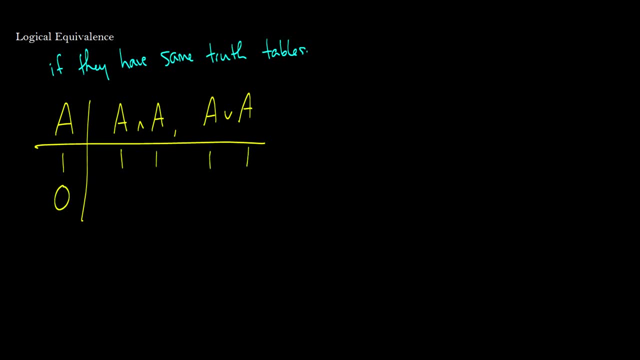 So let's write these out here, underneath all of our a's, and let's see. Let's see what we have here. Well, a and a is true in the first scenario and it's false in the second scenario. and a or a is true in the first line and false in the second line. 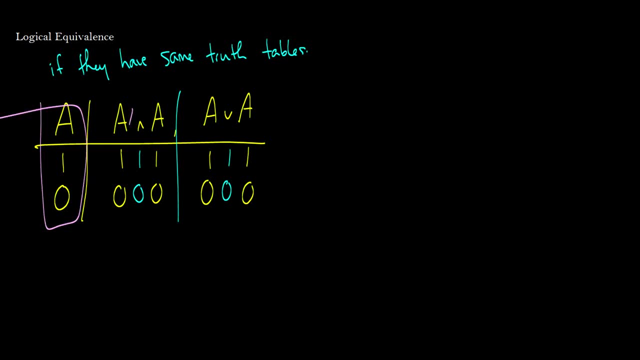 and these all have the same truth tables. Therefore, these are all equivalent and that means that if in a sentence, if you have a, then you can write a or a to mean the same thing, or you can write a and a to mean the same thing. 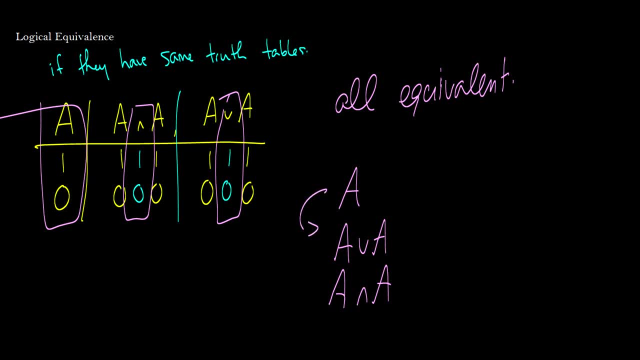 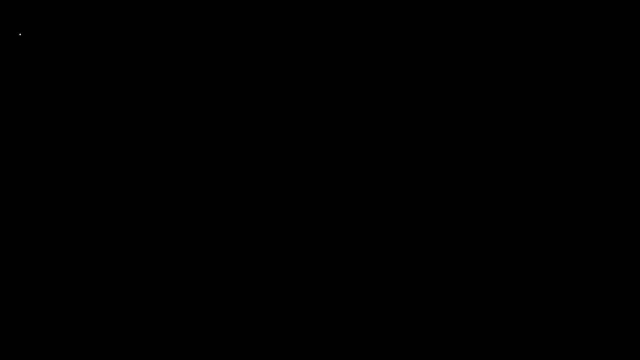 so these are all interchangeable because they all mean the exact same thing. So we're going to do one more, one more. that is very interesting. In fact, I told you before, with the word unless, when we were translating it, that if we have p unless q, this can be the same thing as not q, arrow p or p or q. 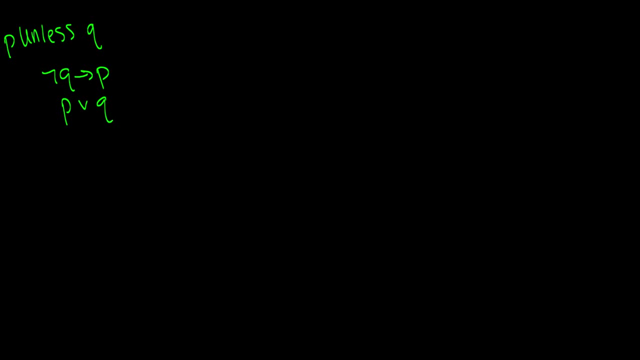 So I told you they were logically equivalent. so what we're going to do now is we're going to prove that these are logically equivalent. So we have p or q here, and we're going to have not q arrow p here. So let's write this truth, table out: We're going to have 1 1 0 0, 1 0 1, 0 for q. 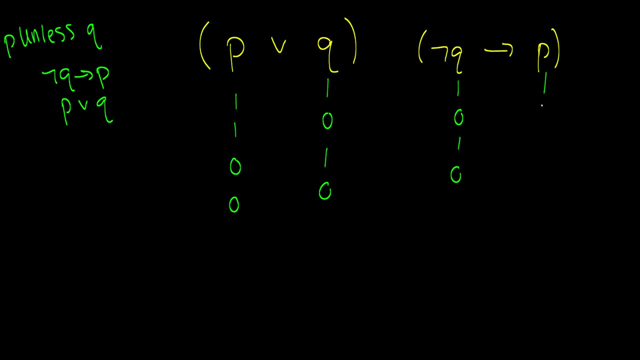 q over here is 1 0 1 0, and p is 1 1 0 0.. Make sure the assignments of numbers are consistent between your two formulas. That should be a given, but I have seen one mistake before. 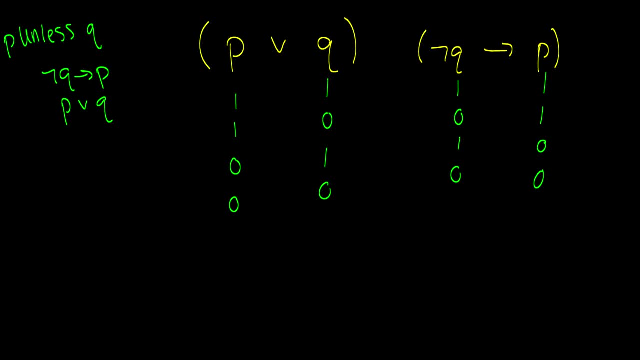 where this happened and it was not pretty because they just couldn't grasp the concept of it. So here we go. p or q is true in all scenarios where they are not both false. so we have a 1 1, 1 0,. 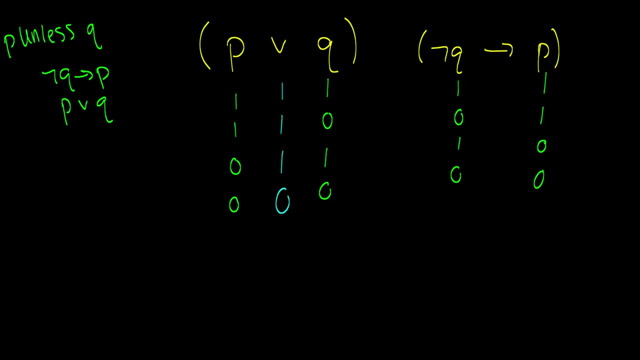 and the second one is only false when the consequent is true and the antecedent is false. but we haven't checked out not q yet, so we need to deal with not q first, And now, in the first line, the antecedent is false.